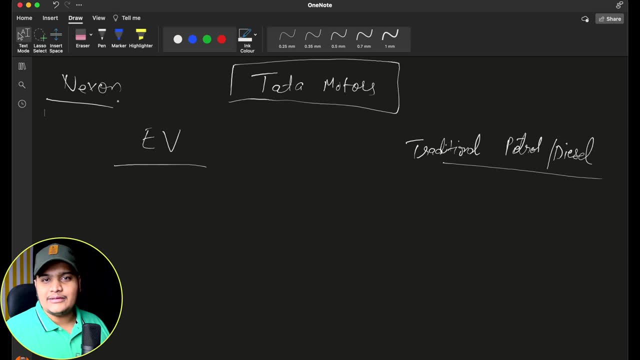 the tata nexon here. So nexon comes in both the variants. it comes in the ev as well and in it comes in the petrol variant as well. So now they decided that they are going to create this nexon in their factory. Now, within the factory, they are going to create the nexon, but for creating 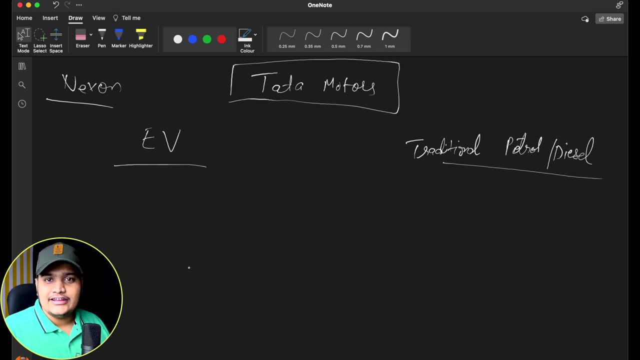 the evs and creating the petrol car, they will need the different spare parts, And the process also should be different, like how you create the different cars. So here let's take the example that within the ev, what you will need is: you will need the motors and you will need 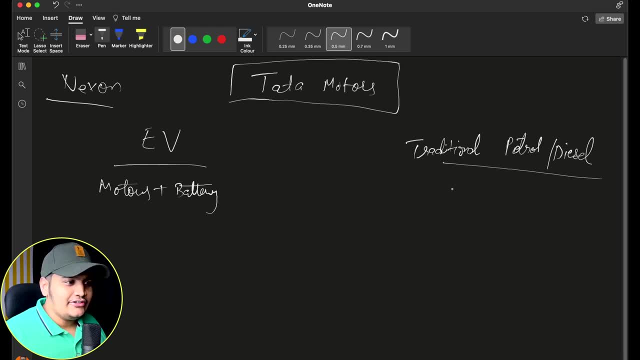 the battery pack as well. But within the traditional car, what you will need is either you will need a petrol engine or a diesel engine. So i'll just mention that either we will be needing the engines and then what we will need is we can need the seats right, But the seats can be same in both. 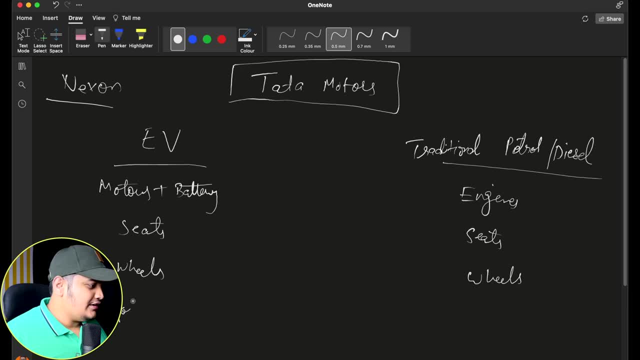 the variants, We need the infotainment system as well, and here as well we need the infotainment system. So infotainment system can also be the same. but you can see that the deciding factor about the two different types of car is just the how you build the engine part or the battery pack. 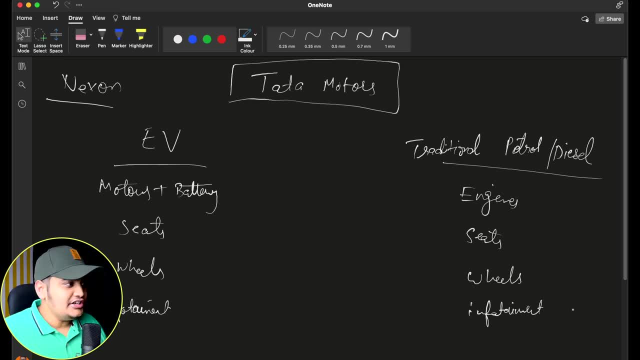 or the motor part. right, Because in the ev you don't need the engine, you need the motors and the battery pack. But in the petrol or the diesel car you need the appropriate engine. either it would be petrol or diesel. Okay, so whenever i want to make a car here, 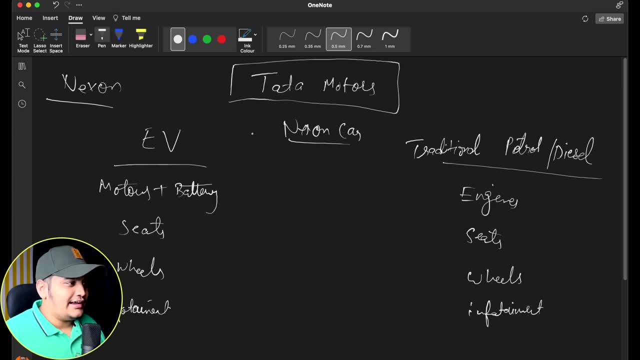 a car. So if i want to make a car, what i can do, what i can tell, that, okay, let's make a car. Okay, and here i can pass. okay, let's either make a ev or either make a traditional car where i will pass the information. Okay, i want to make a car, but it's ev, so i can pass. okay, Make the car with. 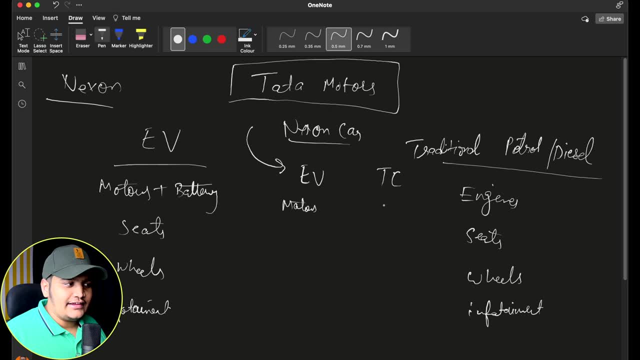 motors or battery pack. Okay, here i can say: make the car with engine. okay, Rest of the things. you can see that those are the default things that we have received before. If you want to make a car, you need to know the engine right So you can use the engine toilet. You can use the engine toilet. 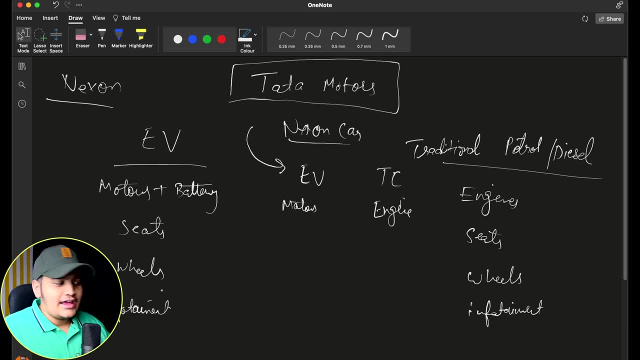 i want to add: okay, i want to add the same seats, i want to add the wheels, i want to add the same infotainment system and rest of the things are everything the same, okay. the only deciding factor changes here: either motors or the engines. so, internally, how it is going to create the ev. 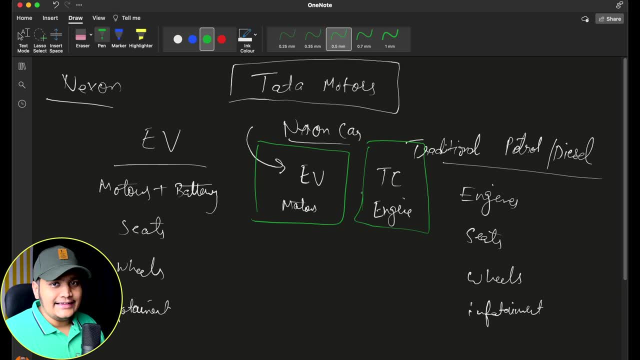 or how it's going to create the traditional engine car, i don't care, i just need the product out. okay, so within the factory, from the assembly process, they can define. okay, is this going to be the ev? okay, so they can define the parameters. okay, rather than engine, put the battery pack and the motor. 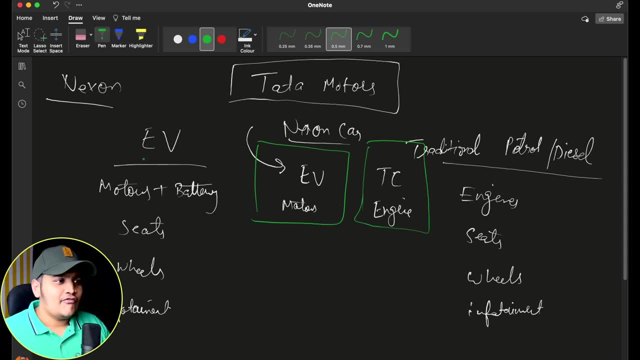 rest everything is same, so rest everything can be in the same assembly line for the traditional petrol rather than the battery pack, and motors keep the engine. rest of the things should be the same. okay, so with this we can design our creation in such a way that, based on some parameters, we can 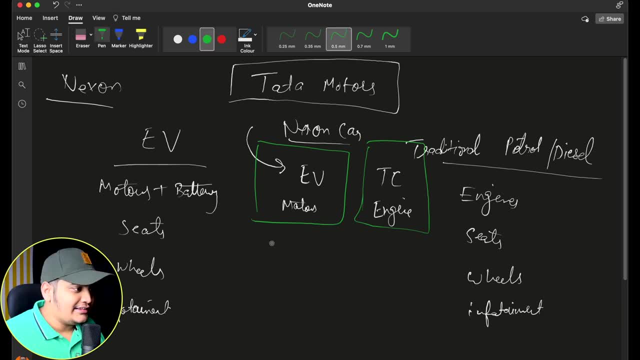 create the objects of it. okay, so, based on the parameters, like either it's going to be the ev or it's going to be the traditional petrol engine car, with this we can create the object or we can create the final product that is going to be the next one car. so you can see. 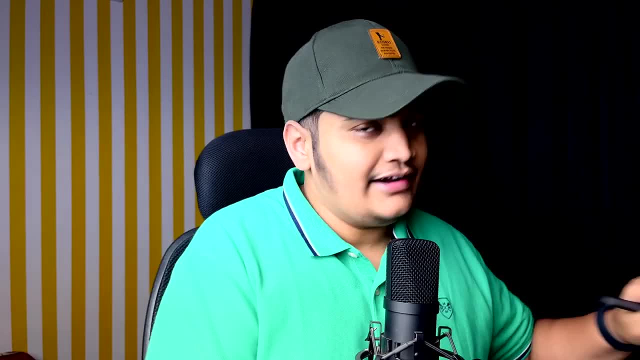 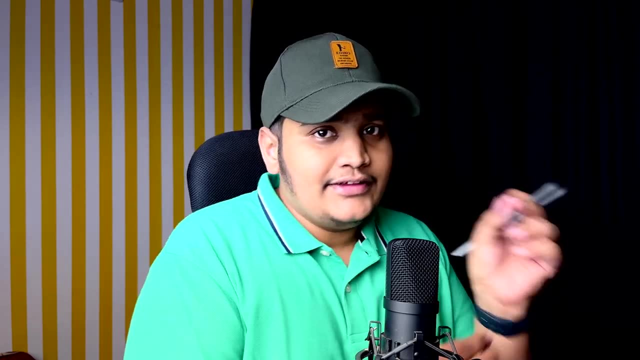 that the creation part. how that particular car is going to be created, that i don't care. okay, that's fine, that's the assembly line that we can create. okay, that they can create. but the idea is based on some parameters. it can internally decide, like, how we are going to create it. 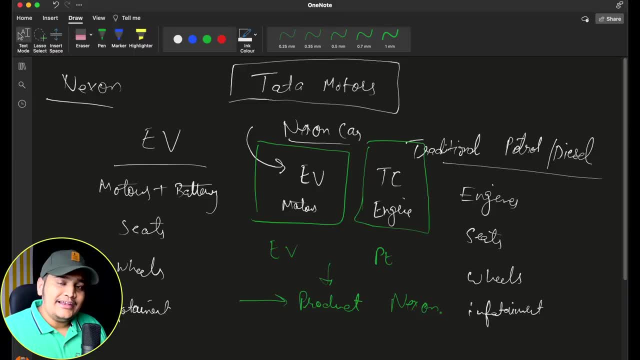 so, within the factory design pattern as well, we are going to decide based on some parameters, like what type of objects that we are going to create. okay, here, if i get the ev as the input, i can create the rest of the things. i can keep it the same for the petrol engine. 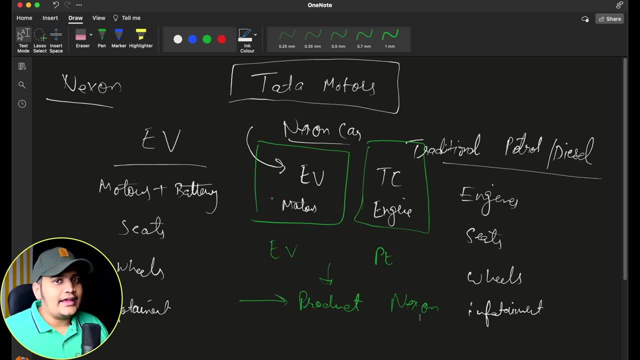 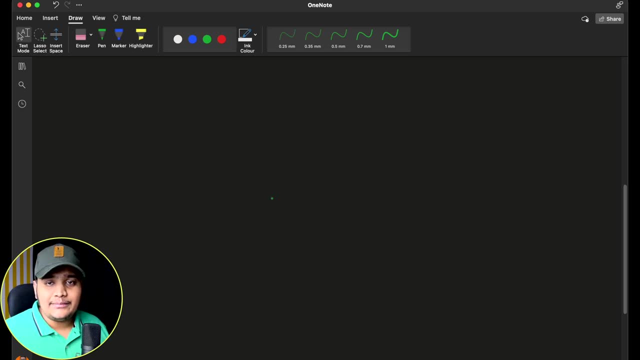 if i get the petrol engine as the input or petrol car as the input, i can create the next one petrol car. so this is how the factory design pattern will work. let's take one more example. suppose you're creating one application and that application can run on windows as well. 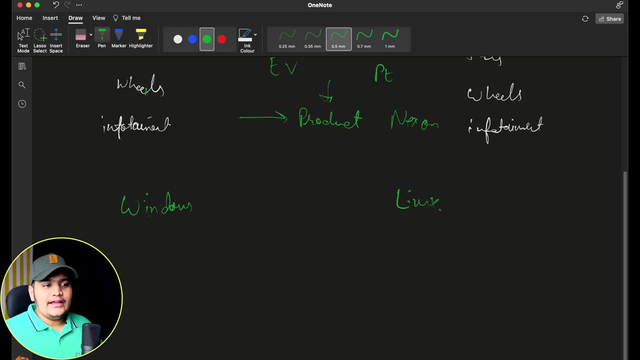 right, and on the linux as well. okay, it can run on both the applications, but we know that the file system in windows and file system in linux is completely different. so whatever the commands that you want to execute, those commands is also going to be different. right, how you handle the. 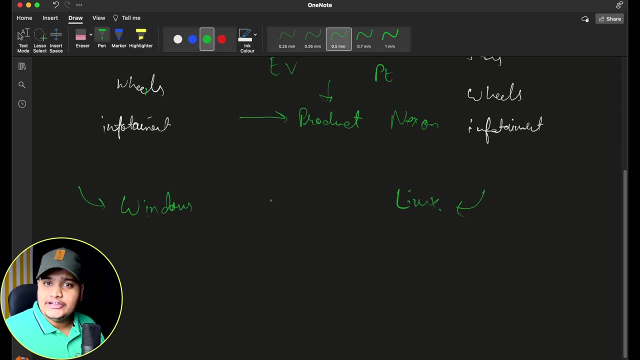 files. in linux, those are also going to be different. now i need to make sure that whenever i am executing those commands, i can execute the commands based on the operating system that has been defined. okay, so if i tell the system that, okay, i am going to run these commands, but on the 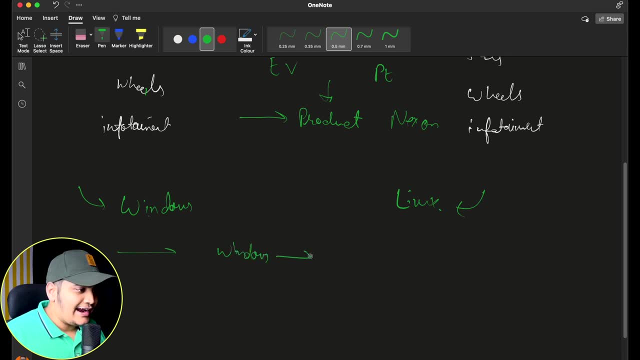 windows. so if i pass windows, okay, i will get the windows object and all the commands which are there and those will be executed directly on the windows itself because those commands will have the implementation for the windows. same way with the linux. if i pass the linux, okay, we will have the linux object created and all the commands defined for that will. 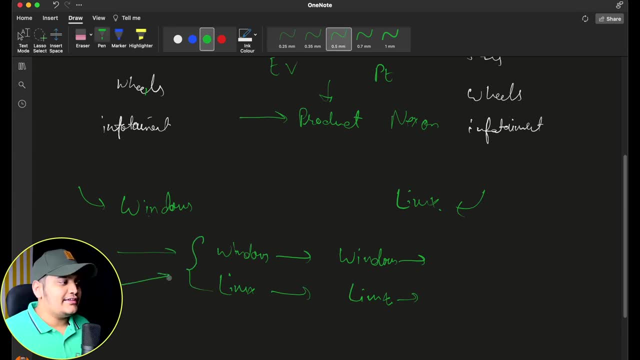 be executed. so you can see that, based on some parameters, we are creating the objects of it. okay, and based on the objects, everything should work accordingly. so that's how the factory design pattern behaves. so let's take this same example and let's understand more. so here you can see. 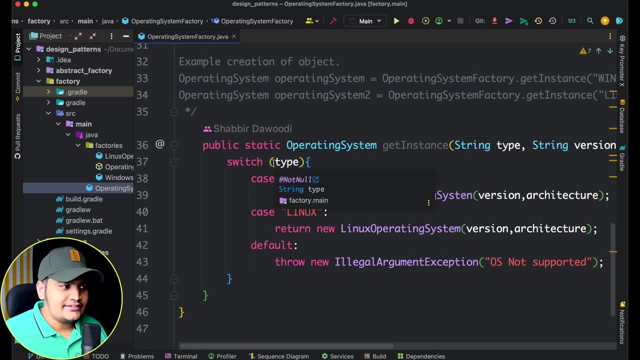 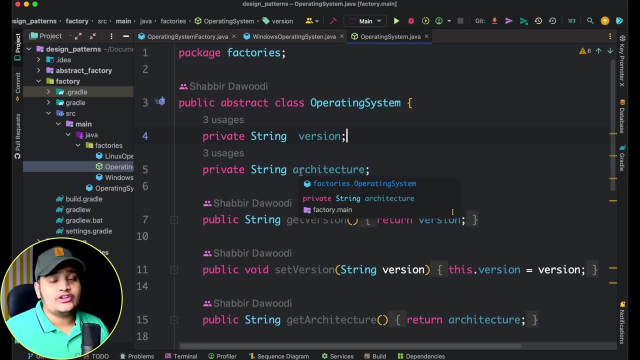 that i have the example here, okay, and i have the example of the operating system and i have multiple operating systems. so here you can see that i have created the abstract class and this principle works on either abstract class or interface. you have to create the interface of. 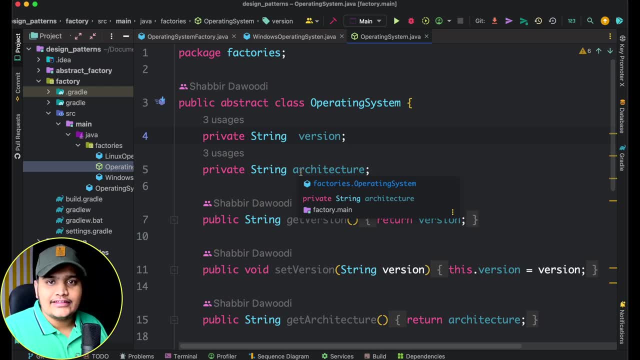 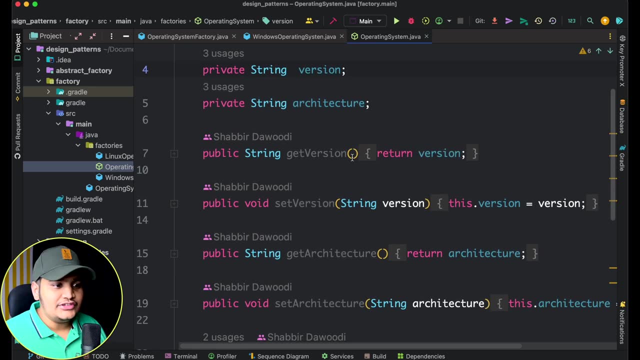 the abstract pattern and the implementation for it. then only we can create the factory design pattern. okay, so here i have created the operating system class. that is going to be the abstract and all the information, which are basic, that we have assigned here. okay, so this is going to have the version. 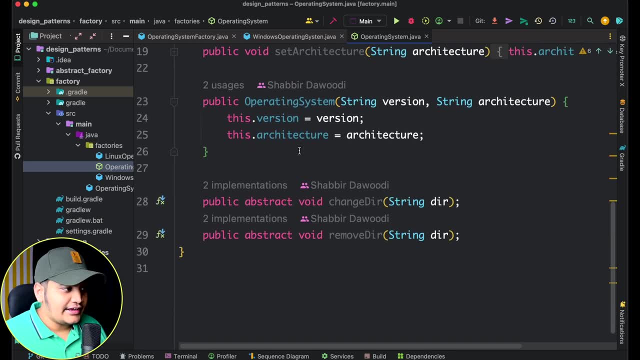 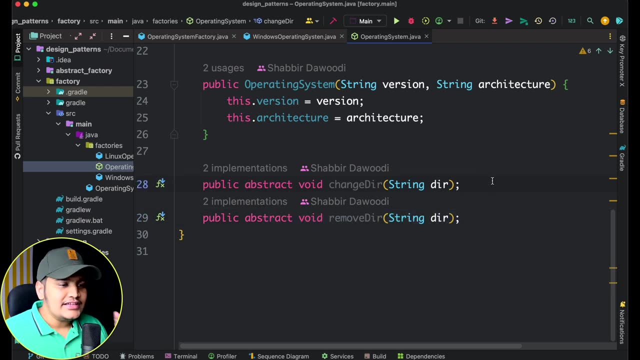 architecture. we can set the version, we can set the architecture type and you can see that the only two methods that we have defined as the abstract methods, that is, the chain directory and the operating system, because these two methods will be different based on the different operating system. so the same thing for the linux operating system, if you go to the linux operating system. 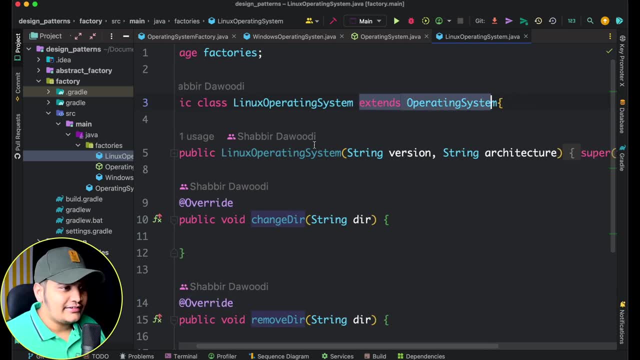 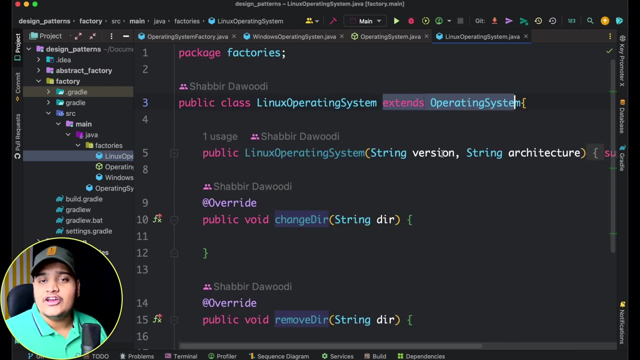 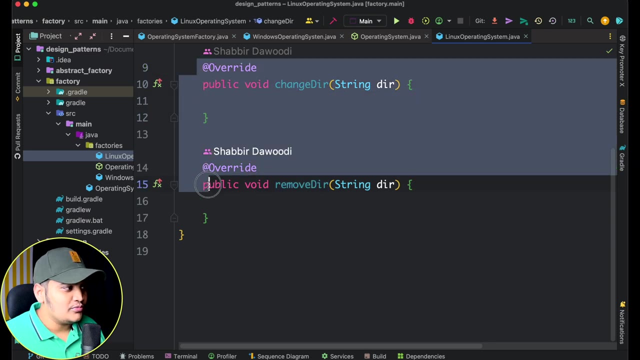 we have defined that is going to be extending operating system, and here we created the linux operating system object based on the version and architecture. that will pass, okay. so whenever i want to create the linux operating system, i have to pass which version and which architecture- okay, and accordingly it will create the object for me, and i have implemented these two methods as well. 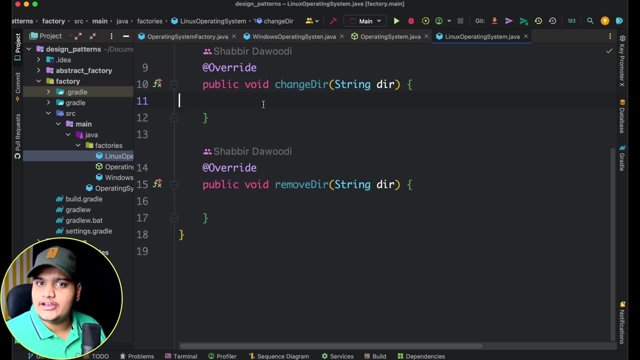 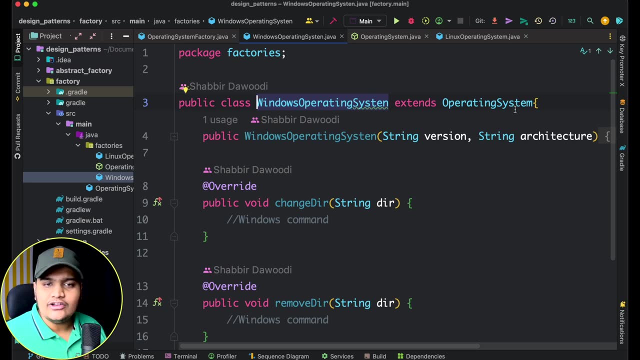 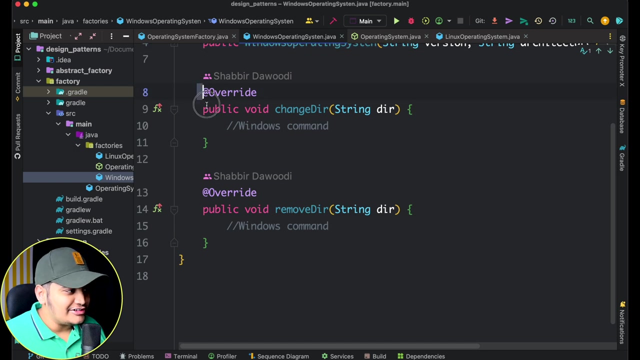 so the command for linux would be different. similarly, if i go to the windows operating system, i have done the same thing. windows operating system will also extend operating system and within the constructor we can create the object but change directory and remove directory will have its own implementation where we can pass the windows command. so this way, you can see, we 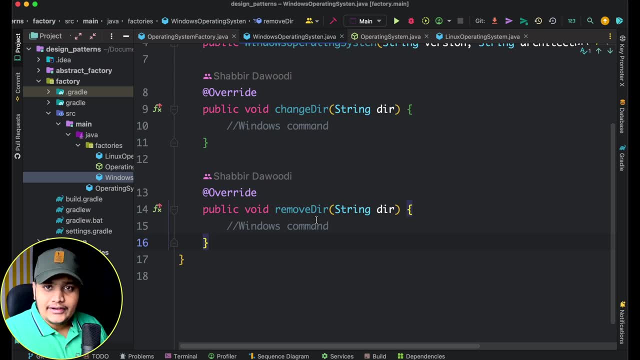 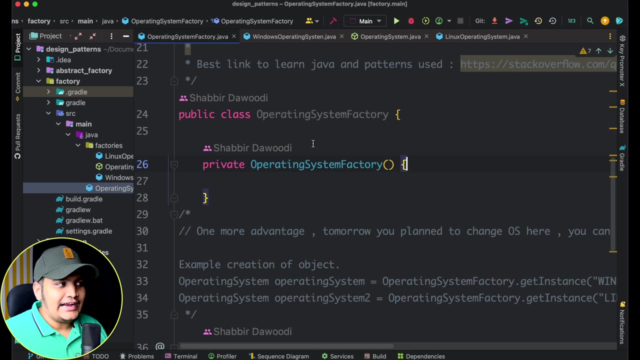 define the operating system and we define linux operating system and windows operating system. both will be extending the operating system and we can also extend the operating system abstract class now how we will be creating the objects. okay, so let's see here. so if we go here, we have created the factory and that factory is operating system factory. now, 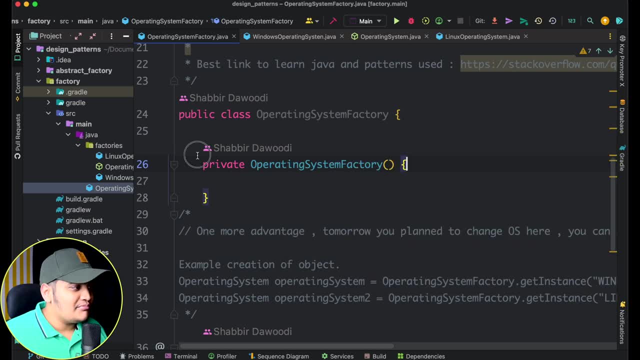 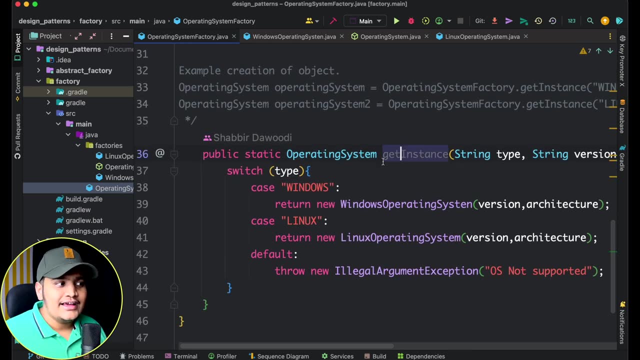 you can see that once we created this operating system factory, we have make sure that the constructor is private. you won't be able to create the factory directly. you have to call the get instance method that is going to return the operating system. okay, ideally you don't need the 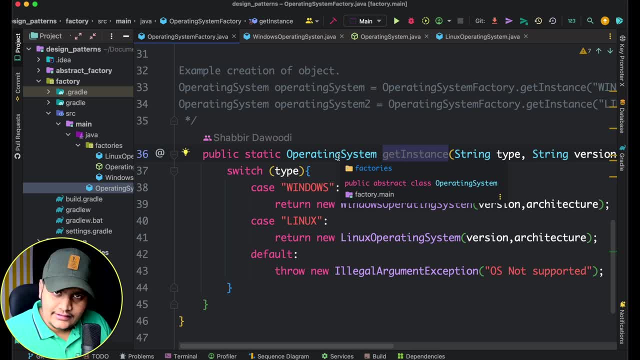 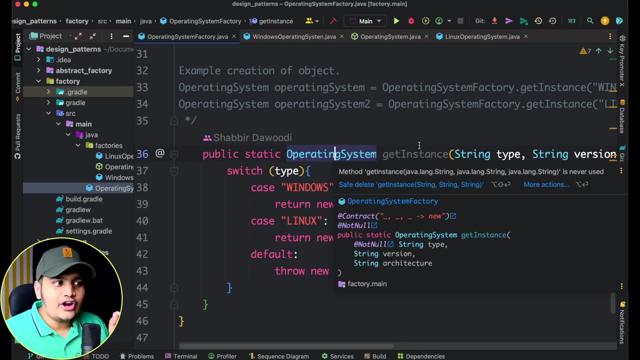 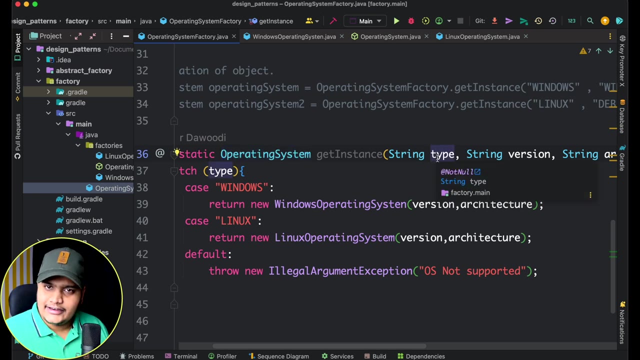 object of the factory. you need the products of it. i need the operating system, okay, rather than the factory. so whenever i am calling this operating system factoryget, instance, in that i will pass what type of operating system i need: either i need linux or windows. that i will pass and i will pass. 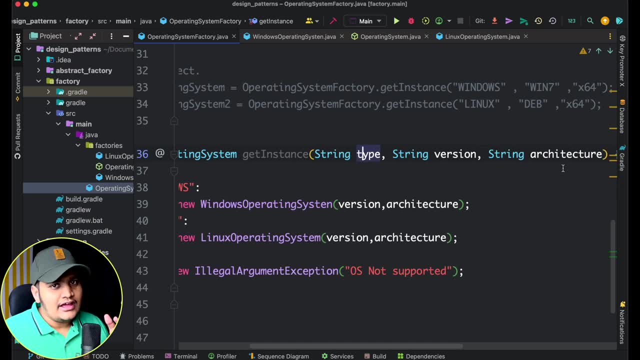 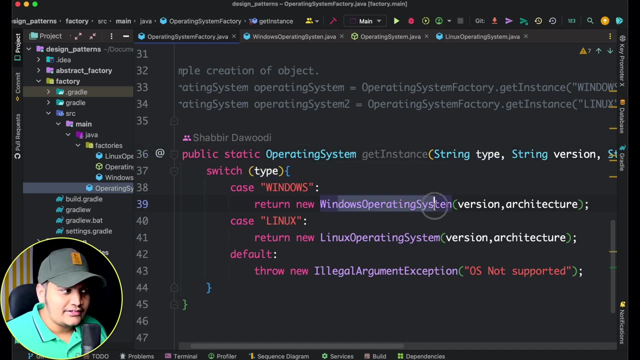 which version i need and i will pass which architecture i need with this three information. okay, with the type itself, it will try to identify. okay, either i have to create the windows operating system based on the windows or i have to create the linux operating system. okay, so you can see. 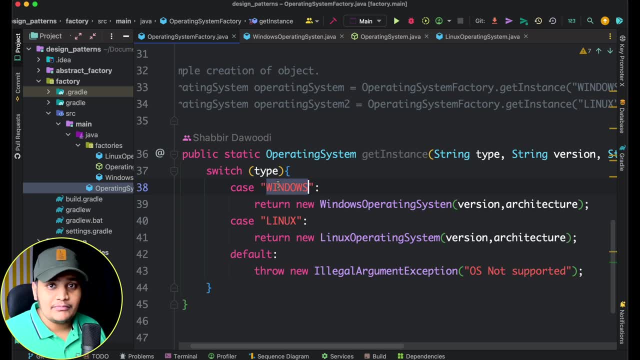 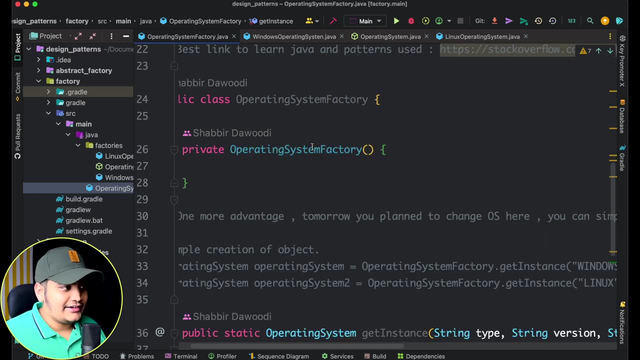 the objects are created based on the parameters that we got, based on some logic or some condition. so accordingly, the objects are created and we got the object from the factory itself. you can see this is the factory and from that factory we got this object. so now you can see we are not directly. 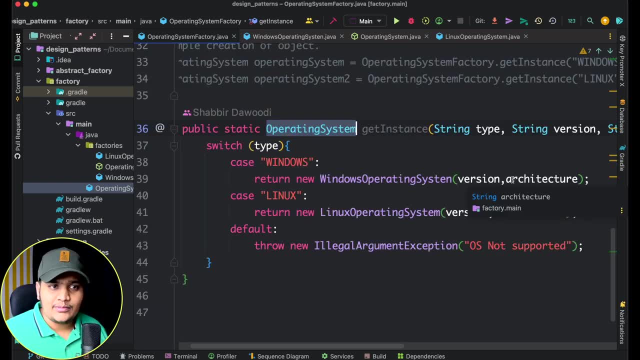 creating the windows operating system object or the linux operating system object. we are just calling the get instance and in that get instance i'm telling: okay, i need windows or i need linux, i need this version and this architecture and get with the object. that's it. we don't have to worry. 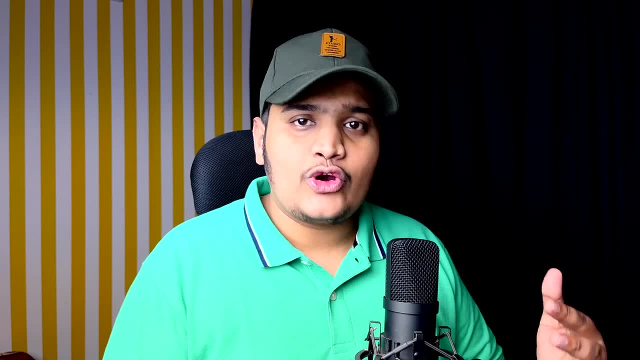 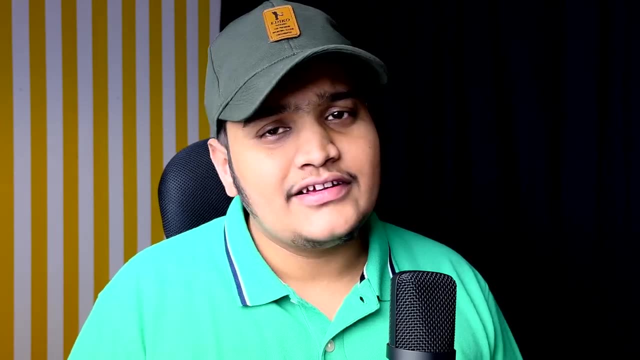 about that. so this is how you can create the factory design pattern based on some conditions. whenever you're creating the object, this is what you can follow. so these are the questions asked a lot in the interviews, so make sure that you know all this easy design pattern as well. so, whenever 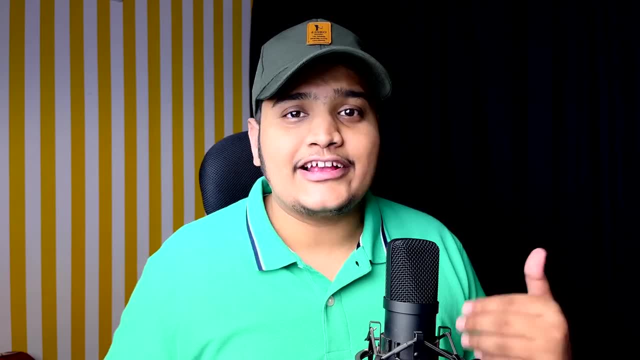 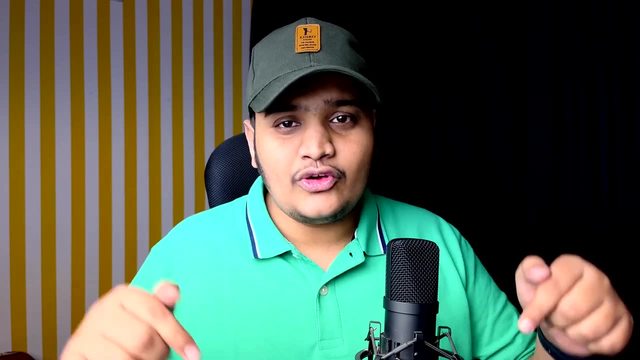 you ask, like: what are the different design patterns that you know? make sure that you know all this so you can explain. so make sure that you at least know one from each categories itself. if you have any doubts regarding any of the things that we have covered, then do let me know. in the 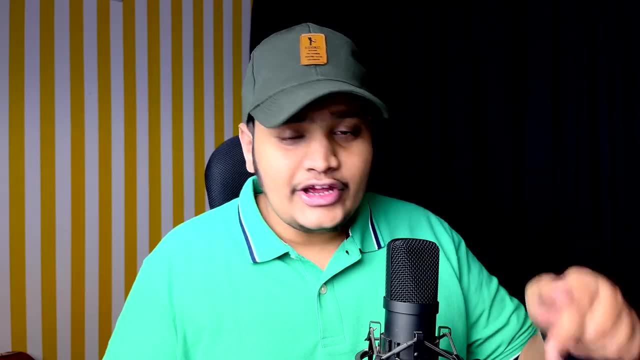 comment section below. if you like this video, give us a thumbs up and subscribe to my channel for the upcoming videos. you can also click on join button to join me on my channel and i will see you in the next video. till then, happy coding, bye.